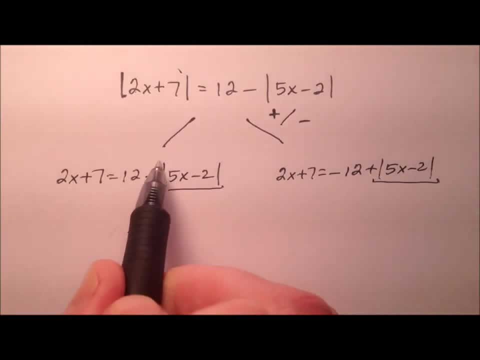 we have the absolute value of 5x minus 2, and it's negative. So let's go ahead and push them over to the left side of the equation and make that absolute value Positive, So 5x minus 2.. And then let's go ahead and take these two terms, the 2x and the plus 7,. 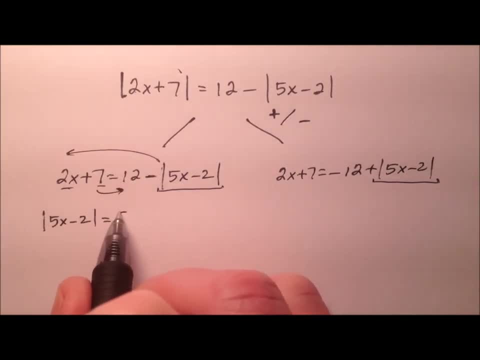 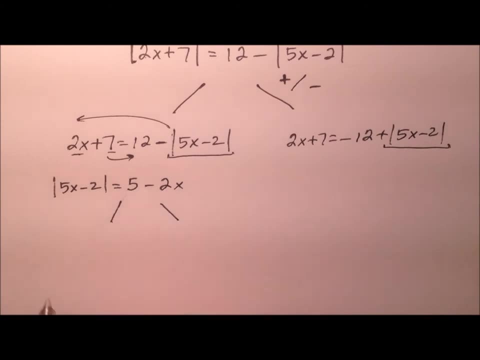 and we'll go ahead and move them to the right side. So 12 minus 7 is 5, and then minus 2x. And while we're over here, let's go ahead and split this up into their two equations, So we'll have the 5x minus 2 from the absolute value here, And then the right side. 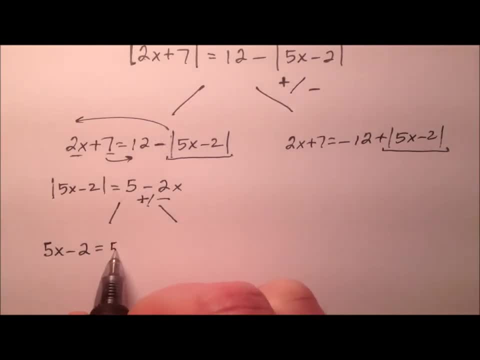 we'll have to take a positive version and a negative version. So we'll say 5 minus 2x and the other one will be: 5x minus 2 equals negative, 5 plus 2x. So let's go ahead and solve. 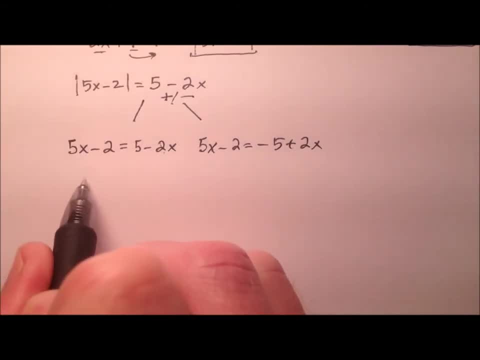 both of these while we're over here. So let's add 2x to get 7x and add 2 to get 7.. So in this first one, x equals 1.. In the second one, here let's go ahead and subtract 2x to give us 3x, and then 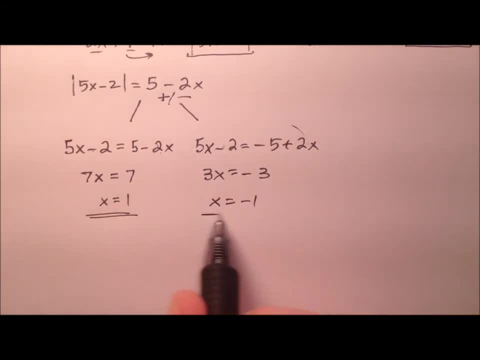 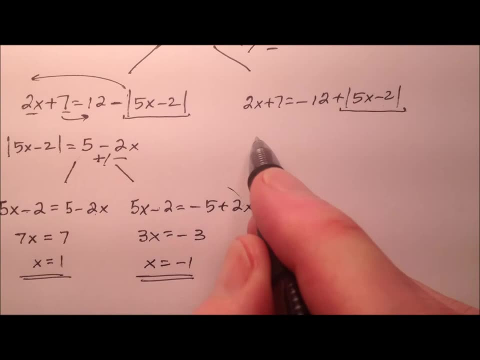 we'll add 2 to give us negative 3.. So x equals negative 1.. Okay, so two pretty easy values here. So let's move away from here and we'll come back here in a second And let's go ahead and focus on this second equation that we had. So here we have. 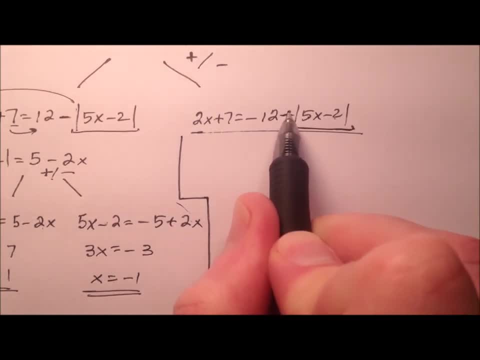 an absolute value. this 5x minus 2 again, but this time he's positive. So let's go ahead and add 12 to both sides, So that'll give us a 2x plus 19 equals the absolute value of 5x minus 2.. 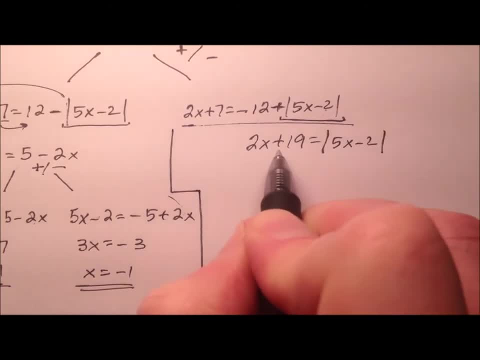 Maybe let's go ahead and use the symmetric property of equality and just switch these two terms. So let's go ahead and add 12 to both sides, So that'll give us a. 2x plus 19 equals the negative 2.. So let's go ahead and add 12 to both sides, So that'll give us a. 2x plus 19 equals the. absolute value of 5x minus 2.. Maybe let's go ahead and add 12 to both sides, So that'll give us a 2x plus 19 equals the absolute value of 5x minus 2.. Maybe let's go ahead and add 12 to both sides. 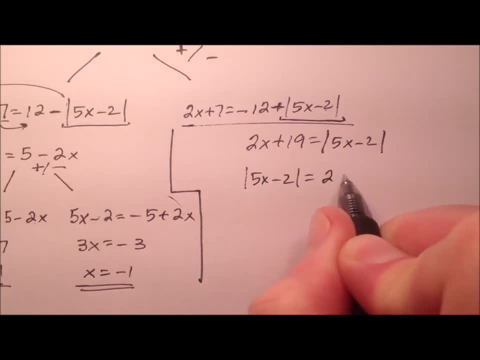 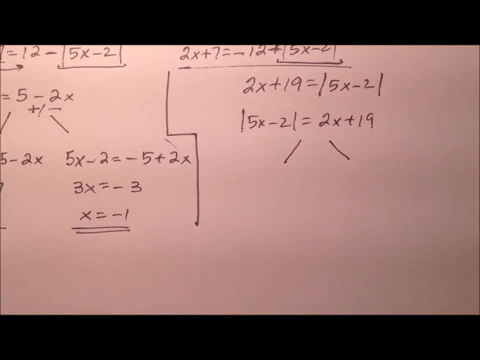 That way we can see our absolute value expression on the left side of the equation. Some people like to see it that way, So let's go ahead and do that. Okay, now it's time to break this up into the two separate equations. So we have our absolute value, which was 5x minus 2.. And to 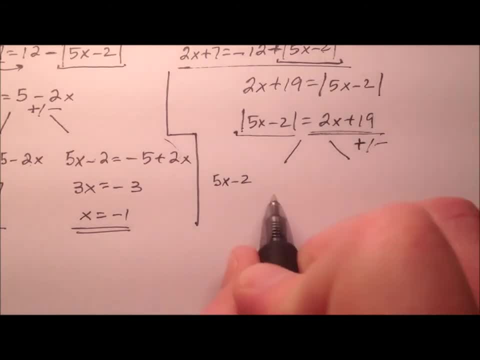 accommodate that on the right side we need a positive version and a negative version. So we'll say 2x plus 19,. and the other is: 5x minus 2 equals negative 2x minus 19.. Okay, let's go ahead and solve both of these equations. So on this first one, 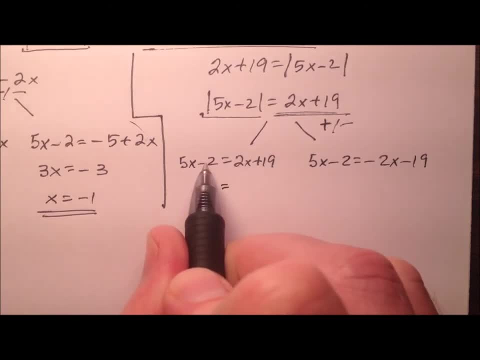 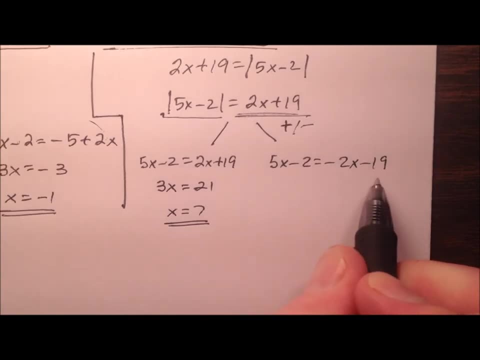 we'll subtract 2x from both sides and we'll get 3x, And we'll add 2 and get 21, and it looks like x equals 7. And that's our third possible value. And finally, we'll add 2x to get 7x. 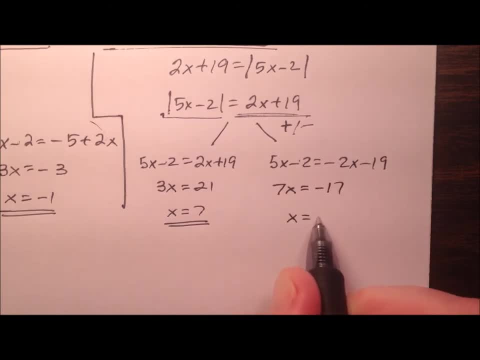 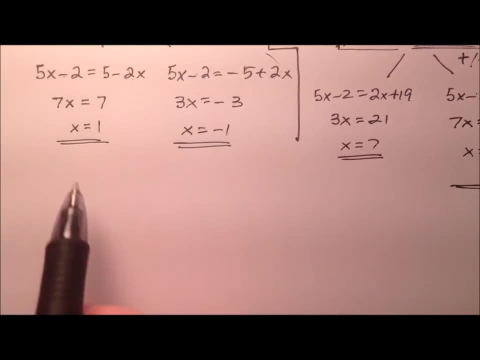 and we'll add 2 to get negative 17.. So x equals negative 17 sevenths. Okay, so here are all four of our values. Let's go ahead Maybe put them together, because I don't think they'll all fit on the screen. So 1, negative 1,. 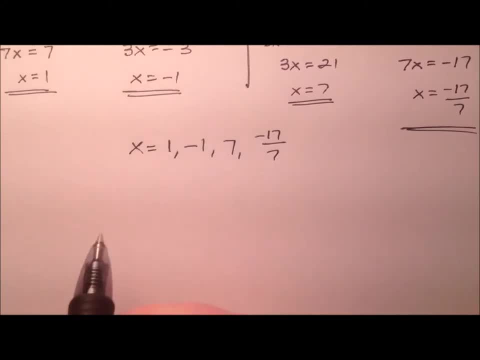 7, and negative 17 sevenths, And I'll go ahead and write our original equation, because we need to substitute all those values back in and see which ones work and which ones are extraneous. Okay, so here are all four values. Here's our original, So let's go ahead and check them. 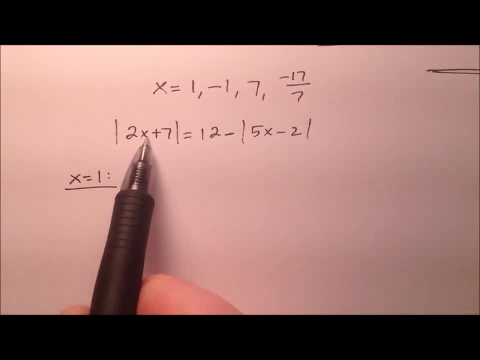 So x equals 1 first. So 2 times 1 is 2, plus 7, is 9.. Absolute value is 9.. So 5 times 1 is 5, minus 2 is 3.. Absolute value is 3, 12 minus 3,. 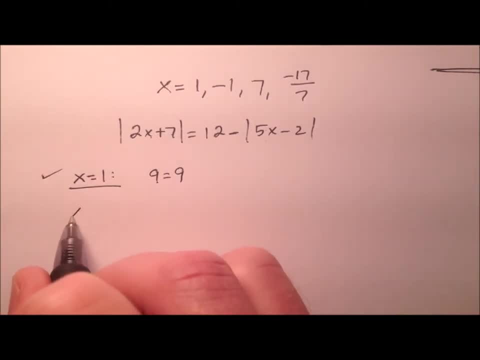 9.. So this x equals 1, it works out, So let's try. the x equals negative 1.. So 2 times negative 1 is negative 2, plus 7 is 5.. Absolute value is 5.. And 5 times negative 1 is negative 5,. 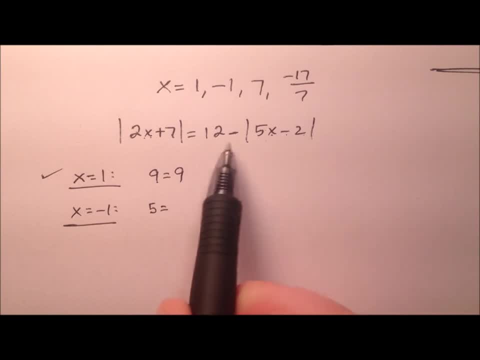 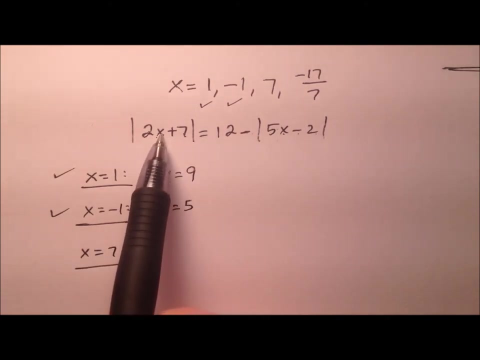 minus 2 is negative 7.. Absolute value is positive 7.. 12 minus 7 is 5.. So we see that both of those first two values work: positive 1 and negative 1.. Well, let's go ahead and try 7 now. Okay, so 2 times 7 is 14, plus 7 is 21.. 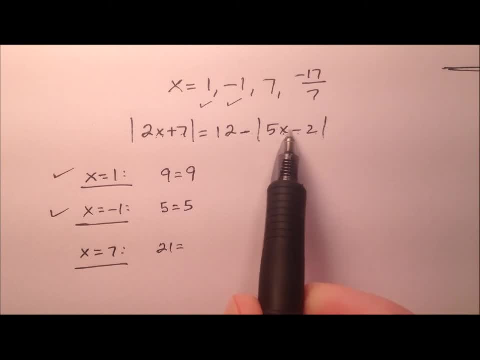 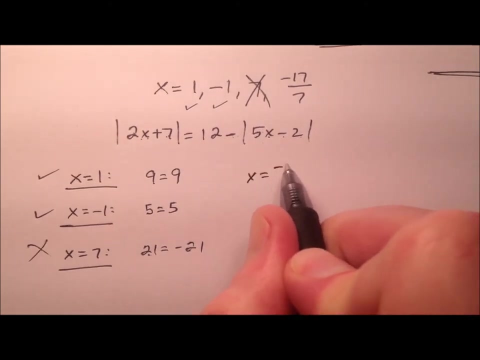 And 5 times 7 is, let's see, 35.. Minus 2 is 33.. 12 minus 33 is negative 21.. So that's a no-go on that one, because 21 does not equal a negative 21.. And finally, let's get a little fraction. 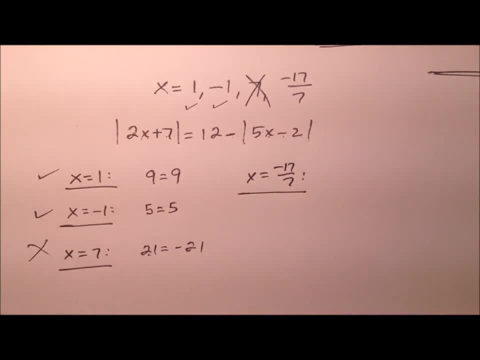 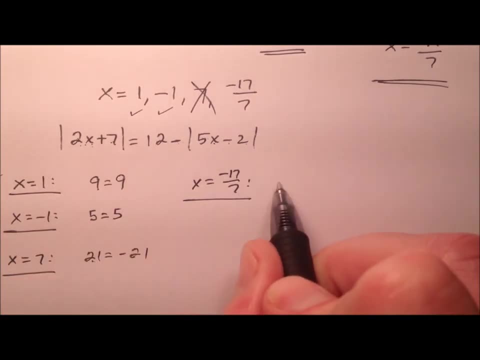 work out by trying: our: x equals negative 17 sevenths. Okay, so 2 times negative 17 sevenths is negative 34 sevenths. When I add 7 to that, I'll be adding 49 over 7.. So that's really going. 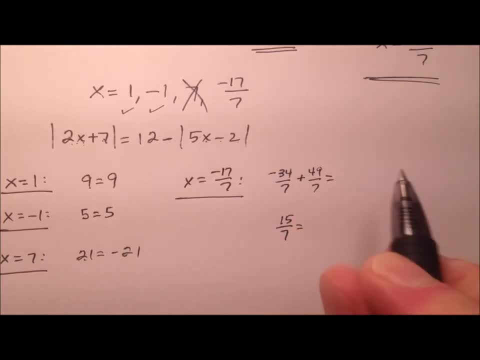 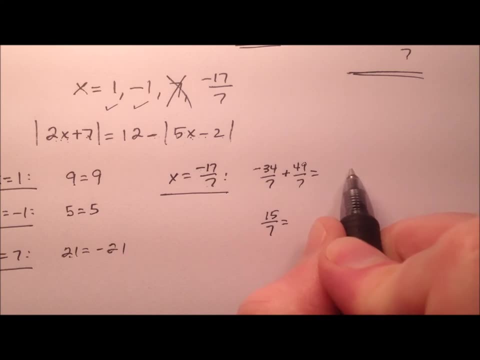 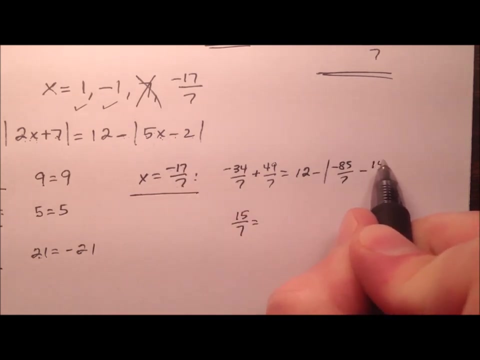 to give me 15 sevenths. Okay, that's the left side. So the right side, 5 times negative 17 sevenths, is negative 85 sevenths, Okay. so let's see 12 minus. we have negative 85 sevenths Minus 2, we'll be subtracting 14 sevenths. So that gives me. 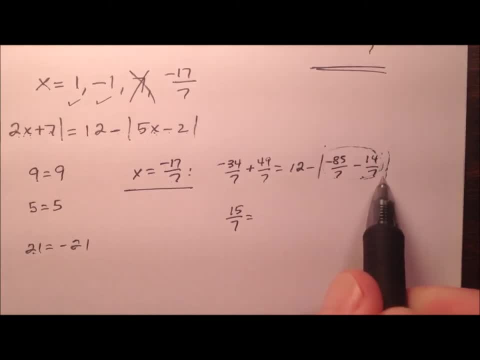 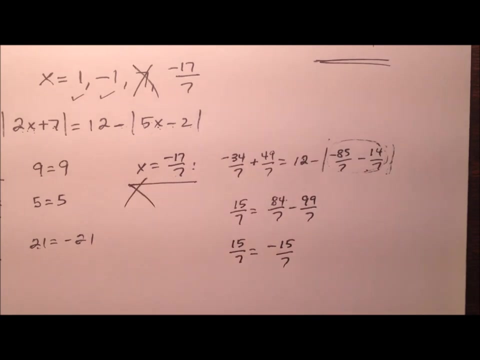 negative 99 sevenths, but it's absolute value, so positive. So when I make this 12 with our common denominator, we have 84 sevenths minus 99 sevenths. So 15 sevenths equals negative 15 sevenths And we can see that that one's a no-go also, so that one doesn't work. 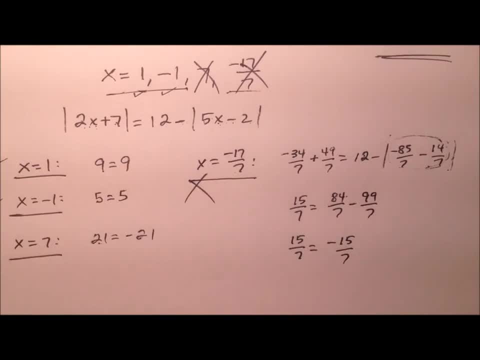 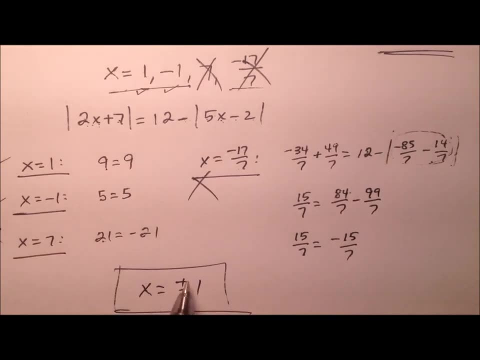 So we had two values that worked and two values that were extraneous. So we can say the solution for this double absolute value equation is: x equals plus or minus 1..